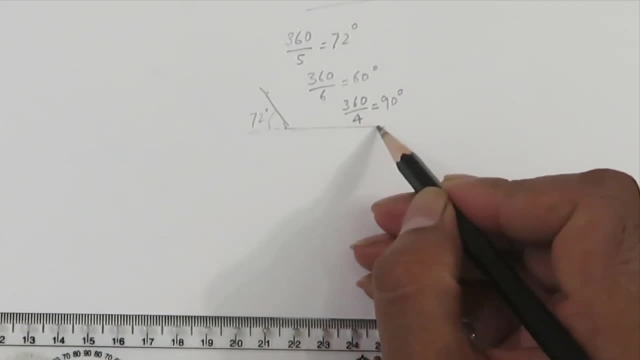 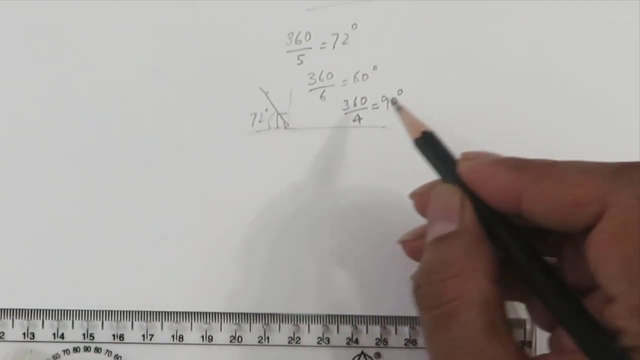 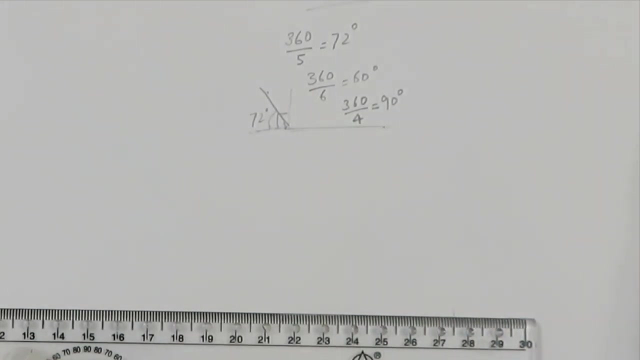 and this gives me 90 degree. so that means first side. the second side will be, will make 90 degree, with the first side on the exterior side. so this is the general rule and we can follow this rule to draw any polygon. but here in this rule, i will show you how to draw. 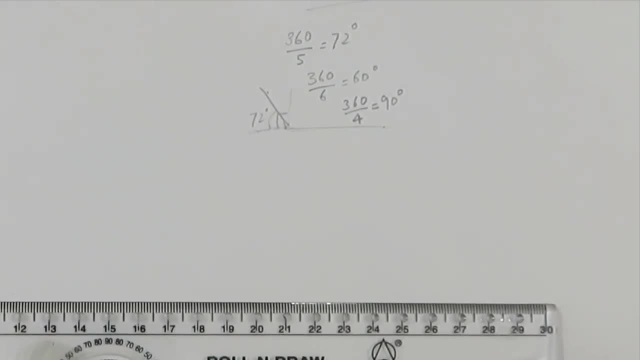 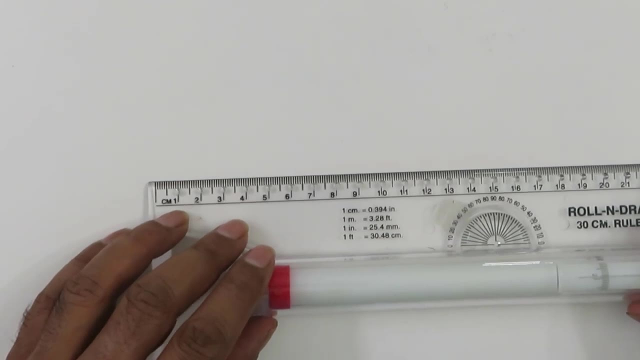 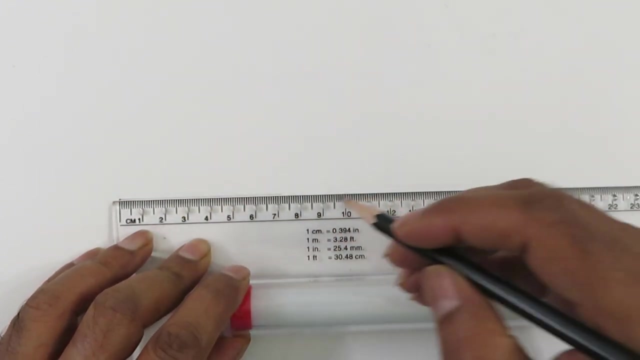 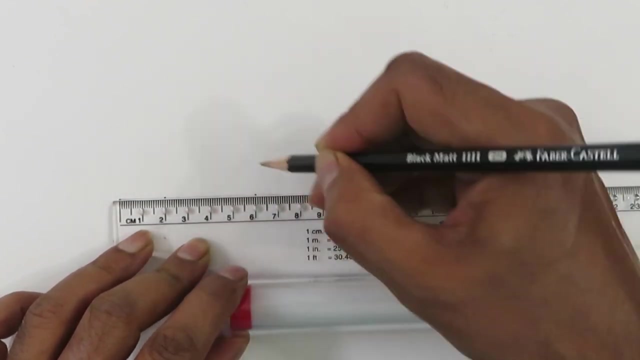 the pentagon and the hexagon, which are quite convenient. so let's draw a pentagon of sides, 40 millimeter. so first we will draw a line and here we will take 40 millimeter. so this is 40 millimeter. this length is 40 millimeter. 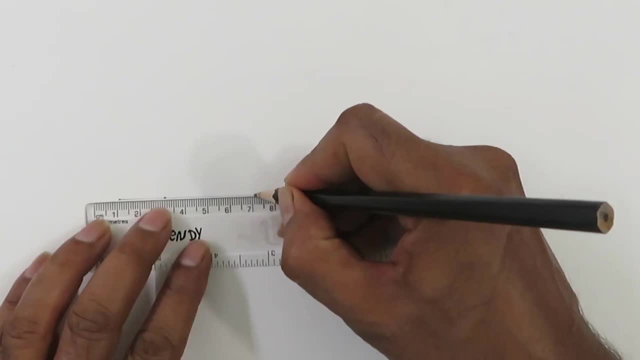 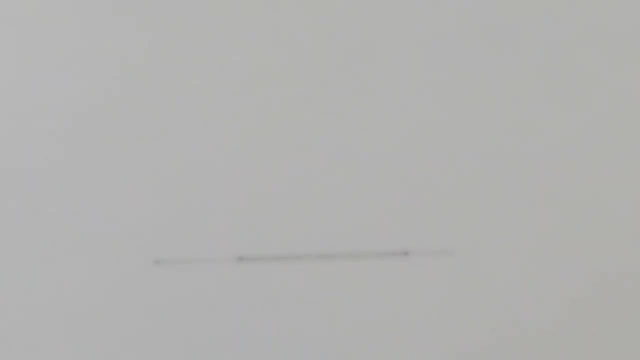 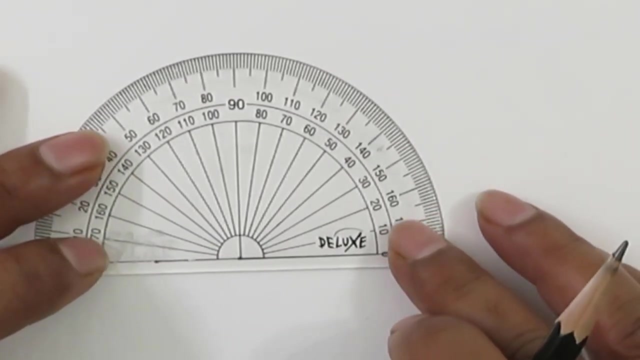 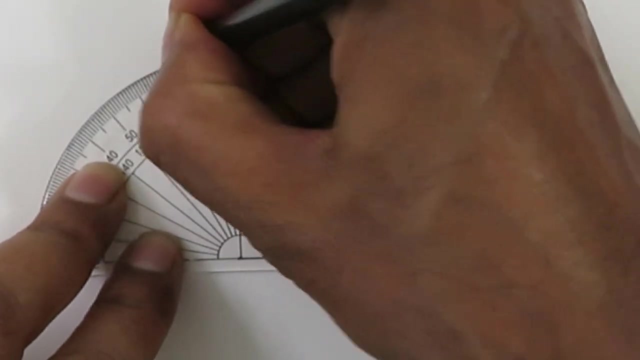 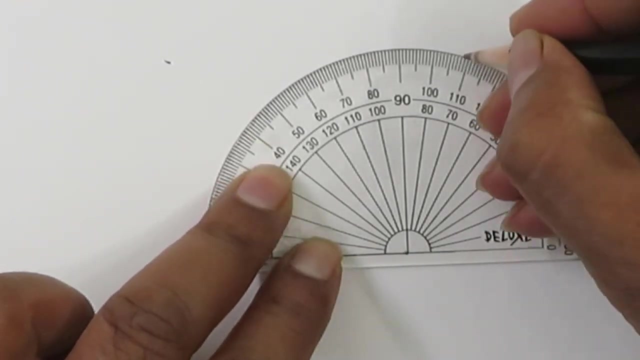 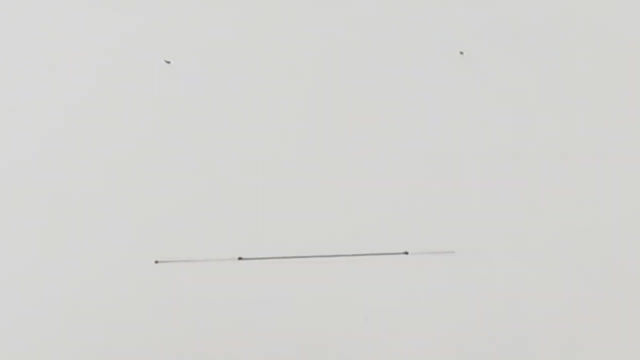 and this is going to be one of the sides. so, since it is pentagon, so we have to make angle of 72 on both sides. you have to be very careful in making this angle again exterior angle, so from here 70. it is possible that we might introduce some error. 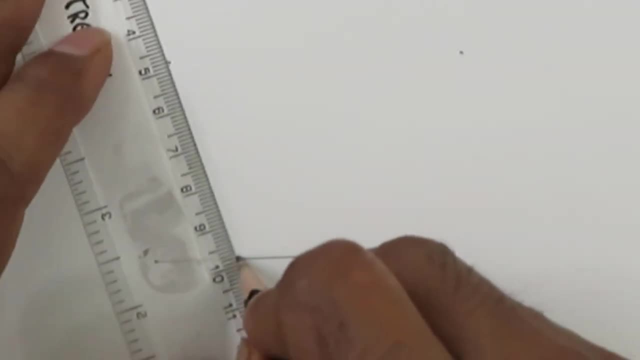 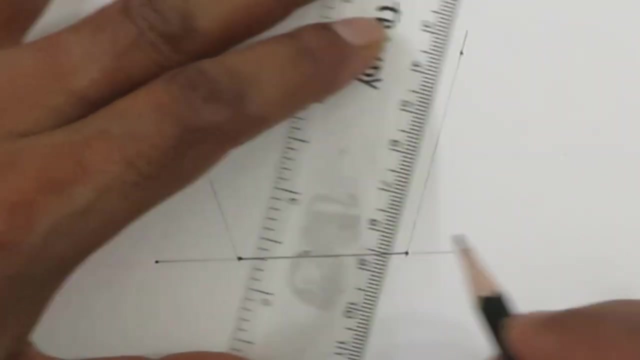 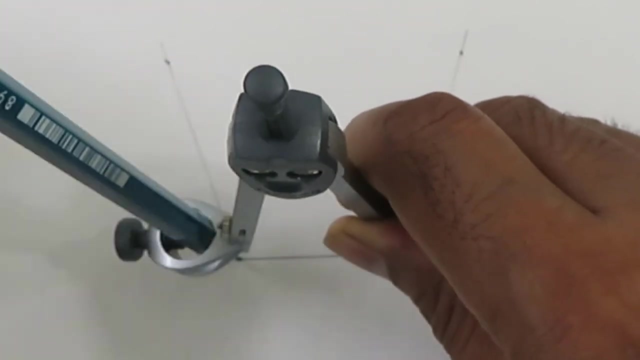 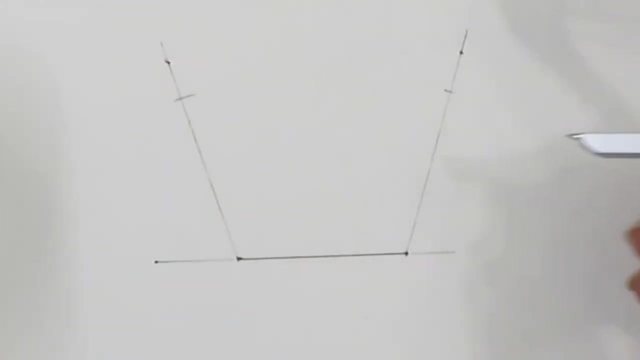 while making the angles. so now you draw a line, a thin line, and you take this distance 40 millimeter in your compass, and then you cut for other sides. so we have about side one, two, three and there has to be two more so we can find out two more by using this compass. so i'm using this compass. 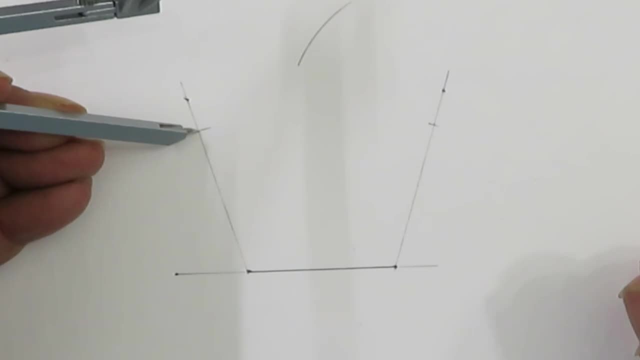 so that we can minimize the error, because there will be some error in measuring the angle. so it's always good to use compass as an example, or as an example of some Breathe angle. these angles are draw not just as an angle, but the distance is also 40 millimeter, which stands 40 millimeter in your compass. 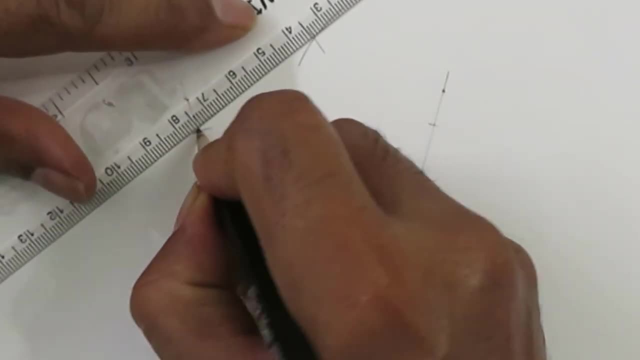 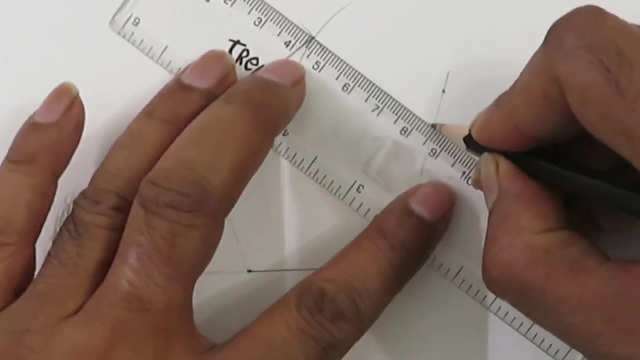 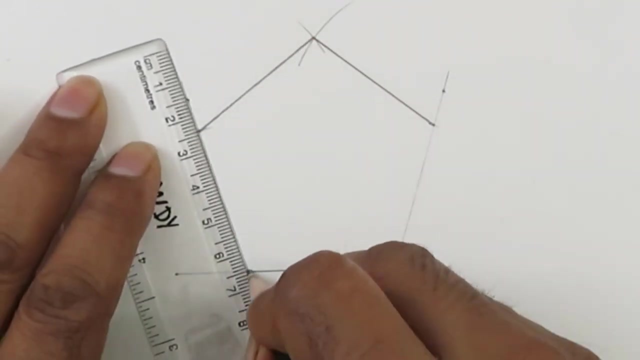 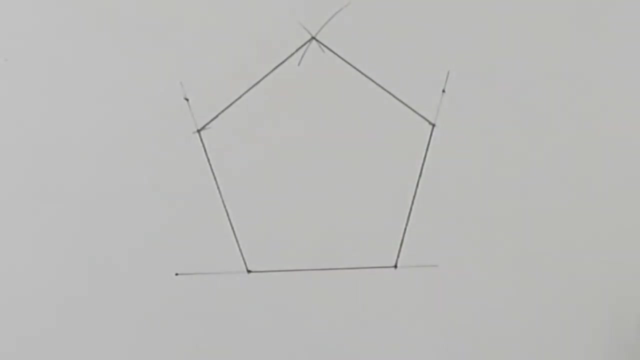 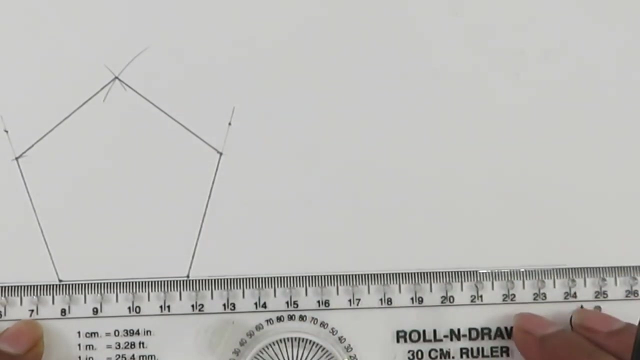 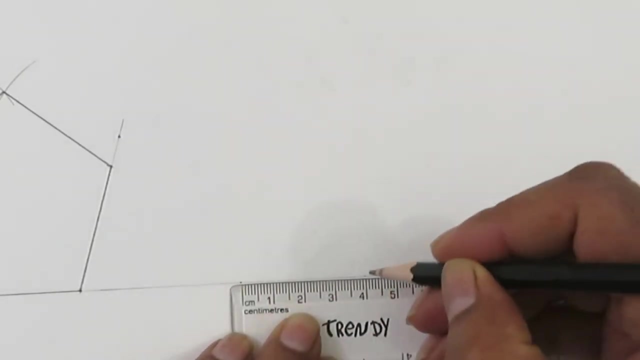 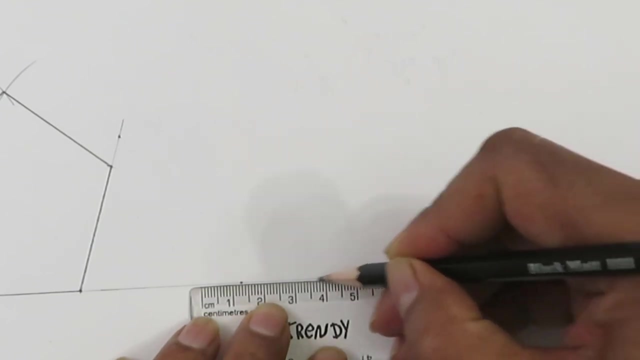 wherever you can. Now, let's darken this line too. So this is the pentagon, and 40 mm is the length of each side. Now let's make hexagon. I just extend on this one and let's take 40 mm. We will darken this line because this is going to be one of the sides of this hexagon. 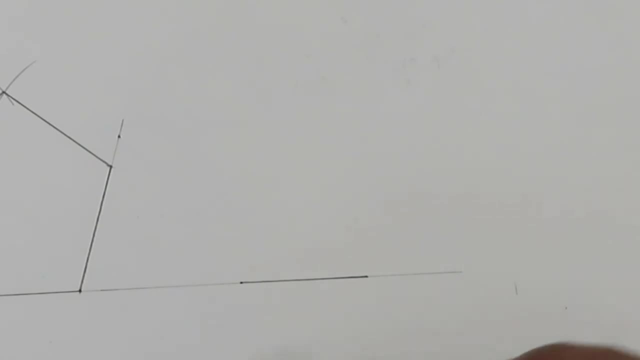 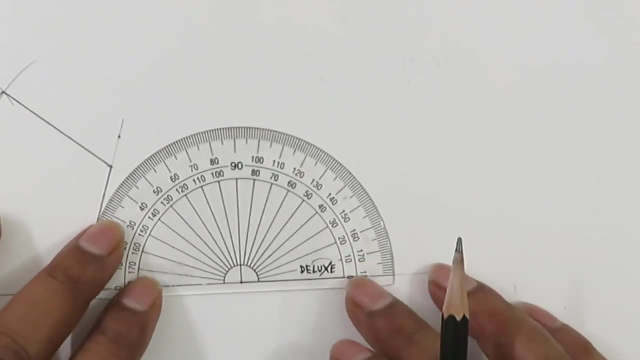 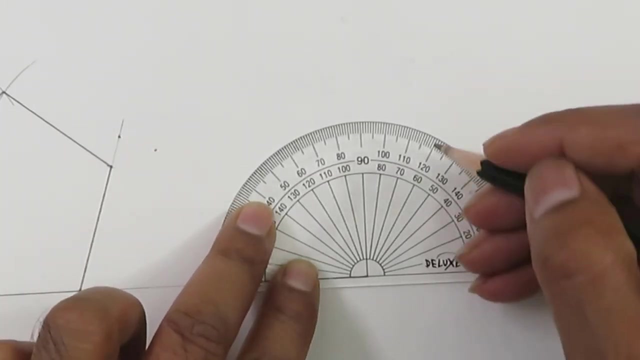 So this is 40 mm And now we should measure the angle And we have calculated that this should be 60 degree. Similarly, on this side, And this is exterior angle, So always know that this is going to be exterior angle, So 60.. 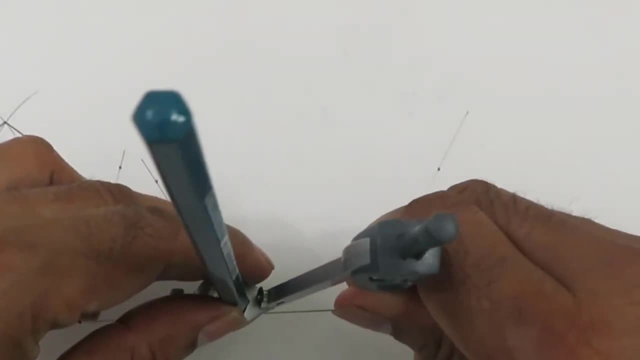 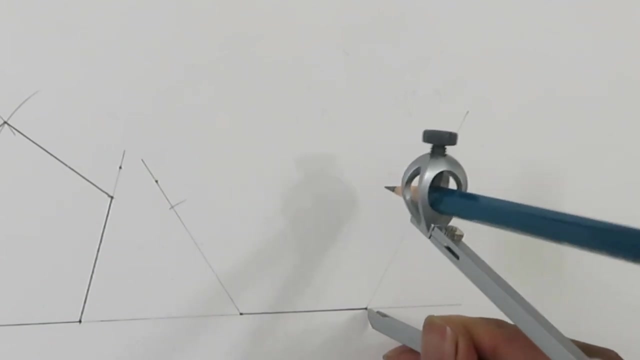 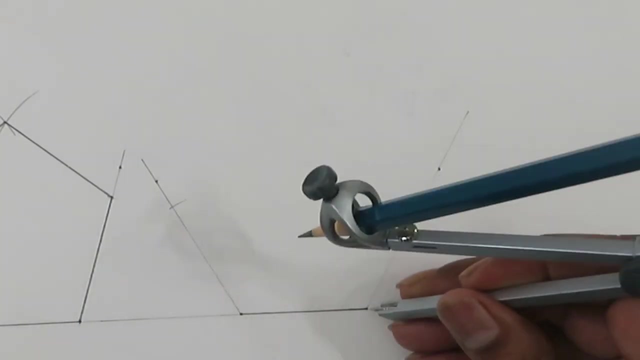 So now again, we will take this 40 mm on our compass And then we cut here and we cut here. So now we have got 1,, 2,, 3,, 3 sides, But we know hexagon has got 6 sides. 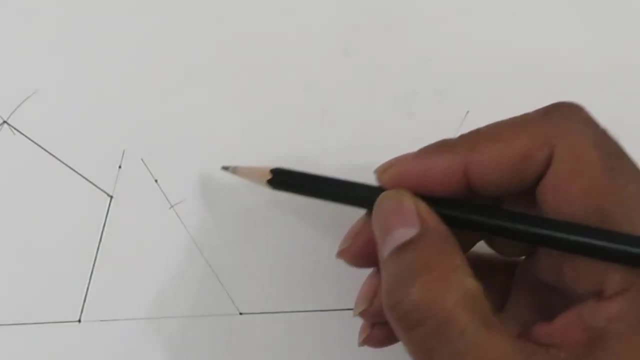 So that means there are 6 sides here, There are 3 sides, 3 more sides, 1,, 2,, 3 here. So now we will take this 40 mm, And then we cut here, And we cut here. 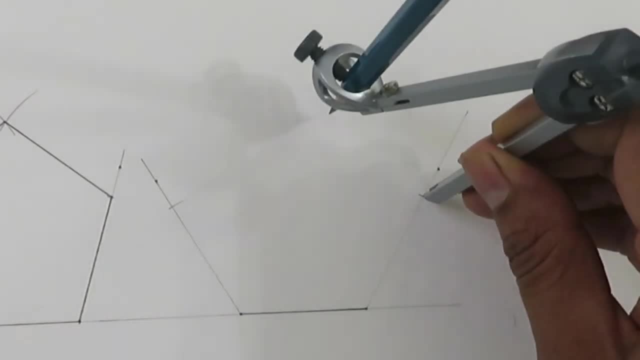 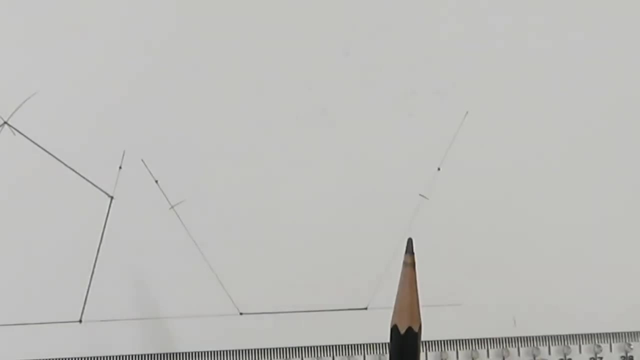 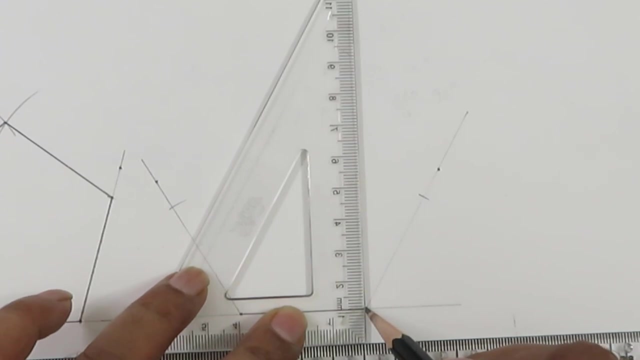 So now, by using this compass, we cannot get 2 points. So therefore, what we have to do is to draw a vertical line. So we should draw a vertical line either here or at this point, And we should draw very thin line, Thin vertical line.